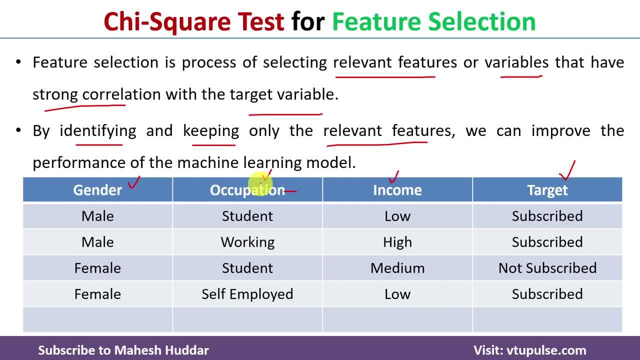 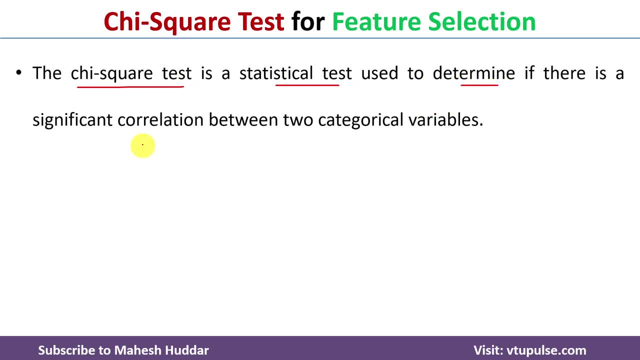 we need to remove it from the data set and we need to keep only the relevant features here. Now we will see what is a chi-square test. Chi-square test is a statistical test used to determine if there is a significant correlation between the two categorical variables. 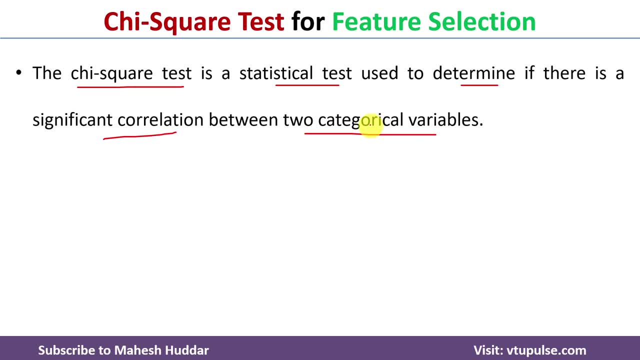 That is, whether there is a correlation between the given feature and the target. we will check it out. If there is a correlation, we keep that particular feature. otherwise we will remove that particular feature from the given data set. Chi-square test is a non-parametric. 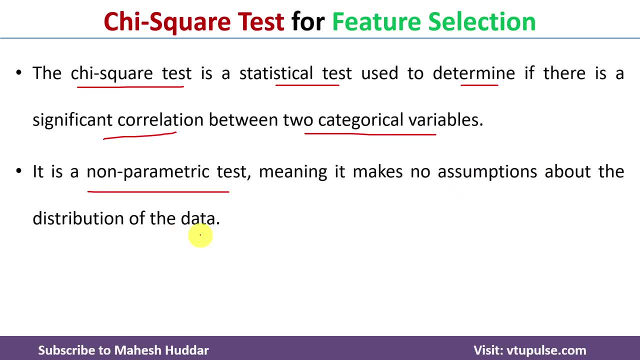 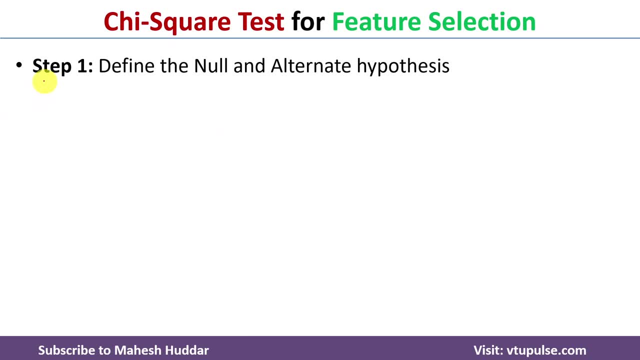 test. It makes no assumption of the particular feature. It is a non-parametric test. It makes no assumption about the distribution of the data. Now we will discuss how chi-square test is used for feature selection in machine learning. In the first step of chi-square test we need: 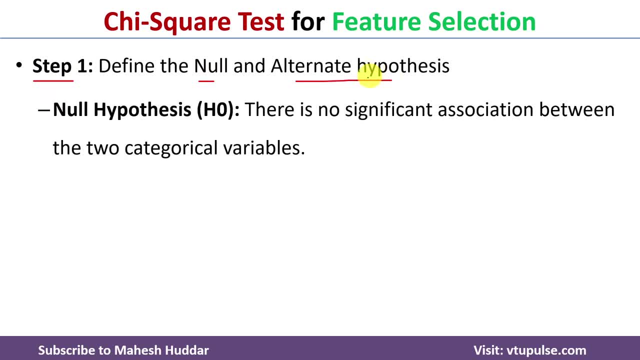 to define the null and alternate hypothesis. here, The null hypothesis, H0, is: there is no significant association or correlation between the two categorical variable. What is the alternate hypothesis, or H1? here There is a significant association or the correlation between the two categorical variable. here 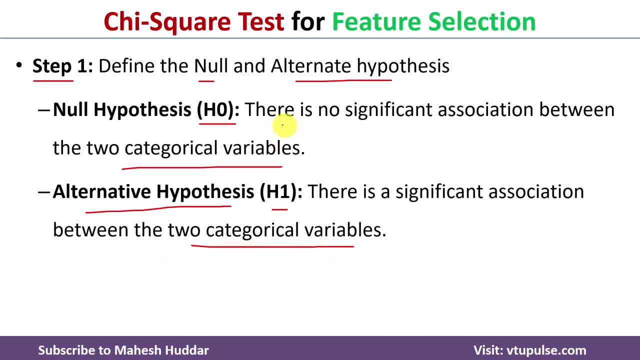 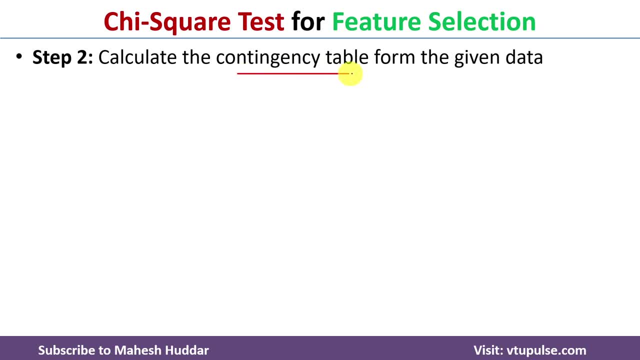 So what we need to do is we need to check whether H0 is accepted or H1 is accepted. in this case, In the second step of chi-square test, we need to calculate the contingency table from the given data. So this is the data given to us. This is just, for example. 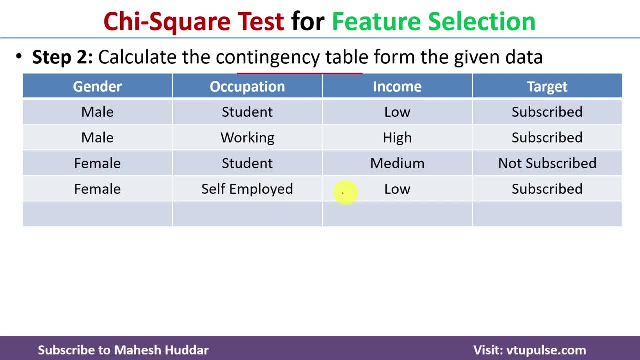 I have taken- This is not the complete data set- here From this given data set. what we need to do is we need to create the contingency table For each of the variables. we need to create the contingency table here. So this is how the contingency table for each. 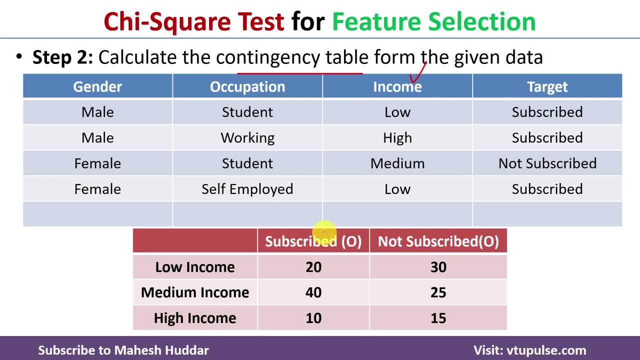 variable looks like The target has two possibilities: One is subscribed and another one is not subscribed, So that's the reason I have taken two columns here. If you have any other possibility in the target, we need to take one more column in this case. And 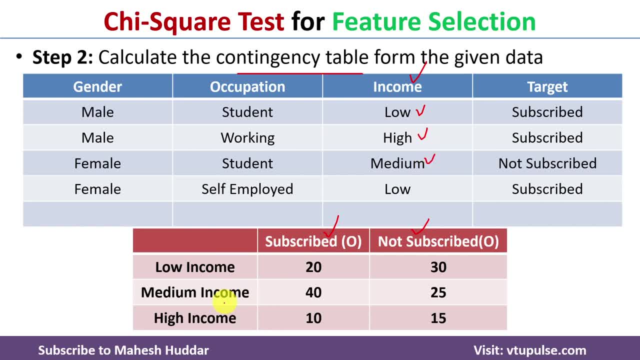 income has three possibilities: low, high and medium. So that's the reason I have taken three rows in this case. Based on the number of possibilities for a particular feature, we need to take the rows. Number of target variables will determine the number of columns. 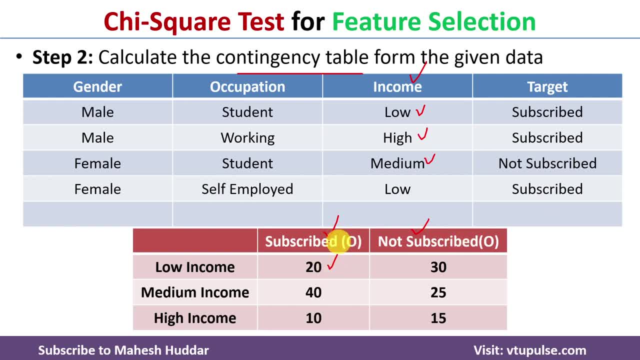 in the contingency table. here We want to get this 20.. So what we need to do is we need to count, whenever there is a low income, how many number of times the target is subscribed. So that is what we need to count In this case. if you count it from the given data, it will become 20. 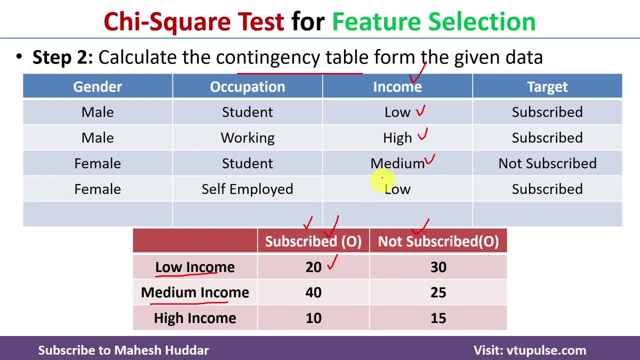 here, Whenever there is a medium income in the income column, how many number of times it is subscribed. That is nothing but this 40 here, The same thing. we have to do it for all other possibilities. we will get the contingency table Again. I will tell you. 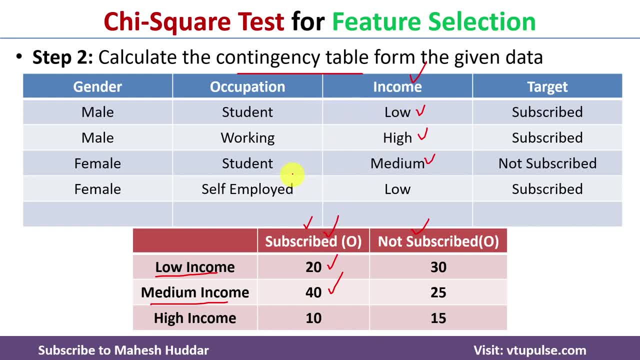 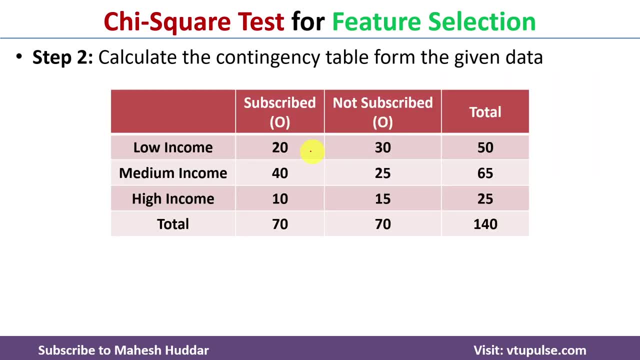 in this case I have not considered the entire data, Just for example purpose. I have shown a part of the given data and I have shown how to calculate the contingency table. in this case, The same contingency table. I have written it one more time. I have added one. 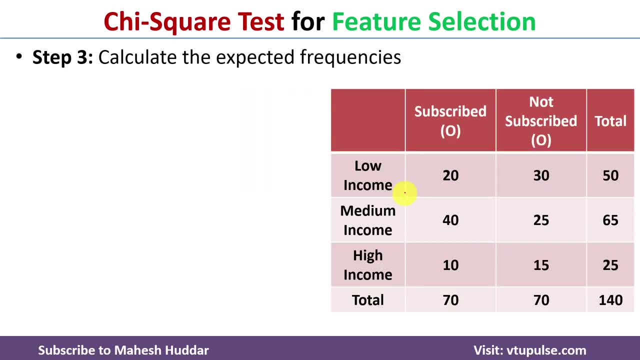 total column and total row in this case. Coming back to the third step, in this case we need to calculate the expected frequencies. We know the observed frequencies. What we need to do is we need to calculate the expected frequencies. here, Now, the question comes in. 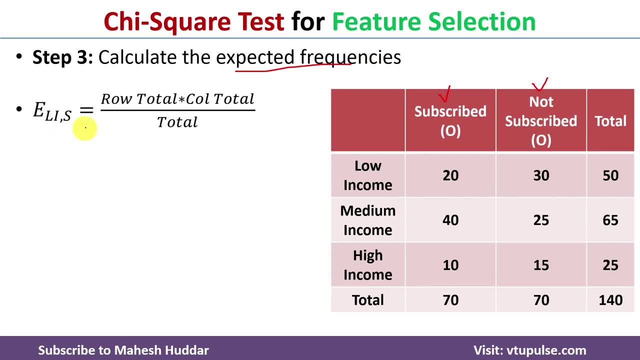 front of us. Let us calculate the expected frequencies. To calculate the expected frequency, we use this formula: The expected frequency of low income given subscribed, that is, low income given subscribed. This is what Observed frequency. I want to calculate the expected frequency. 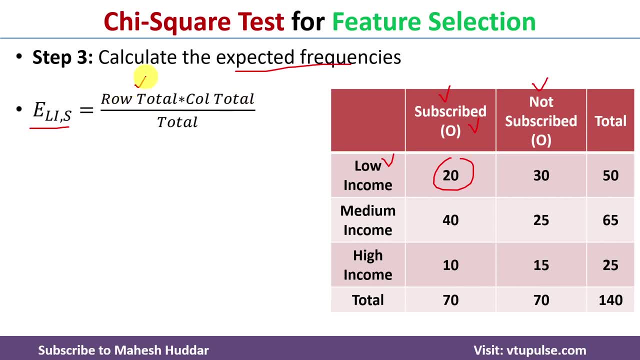 here. That can be calculated using this formula. That is row total multiplied by column total. Row total is how much here? 50.. Column total is 70.. So 50 multiplied by 70, divided by total, that is 140 here. 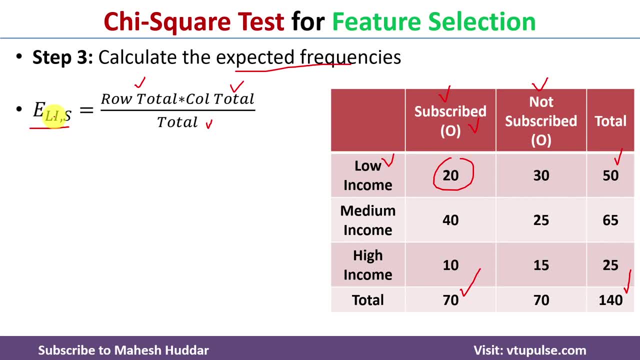 So this is how we calculate the expected frequency of low income given subscribed here. So that is 50 multiplied by 70 divided by 140 is equal to 25 here. Similarly, expected frequency of medium income given subscribed Observed frequency is 40 here That is expected. 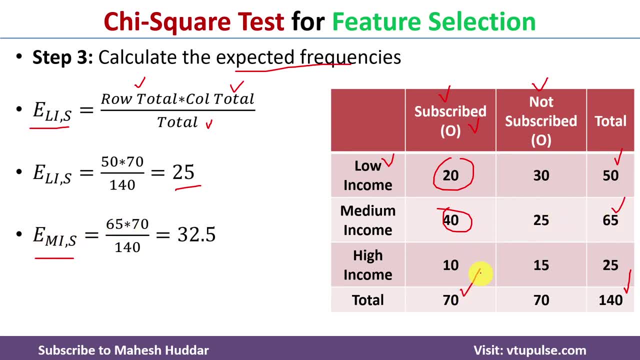 frequency is the row total is 65 here. Column total is 70.. That is 65 multiplied by 70. divided by total, That is 140, which is equal to 32.5. here Now let us use this formula. We have: 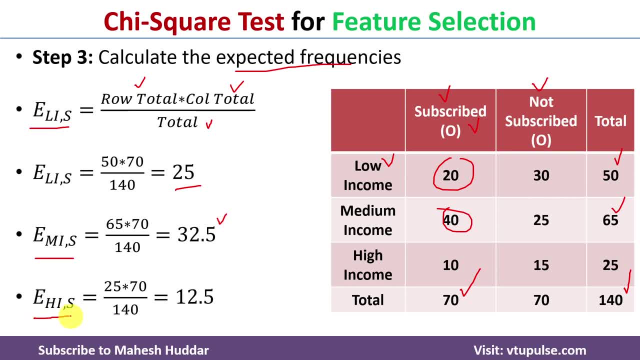 calculated the expected frequency of low income given subscribed. So that is 50 multiplied here. similarly, we need to calculate the expected frequency of high income given uh the subscribed here. so we will get the expected uh subscribed frequencies here the same we have to do it for. 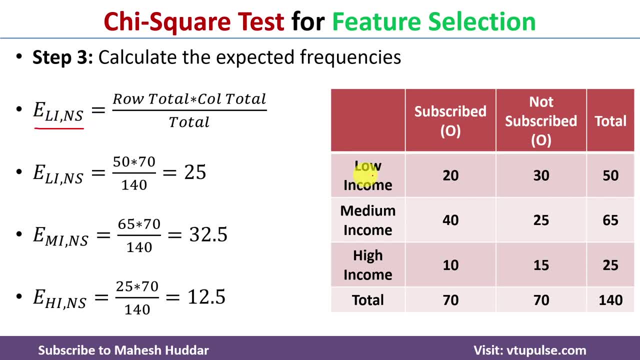 not subscribed. also, that is expected frequency of low income given not subscribed. that is what we need to calculate. that is nothing but the row total multiplied by column total divided by 140. here again, the same thing we will get. that is 25 in this case. the second one is expected frequency. 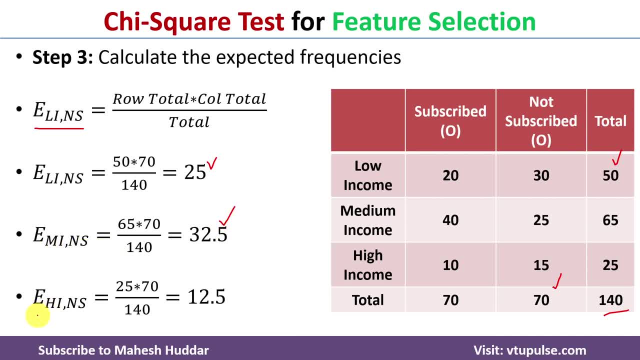 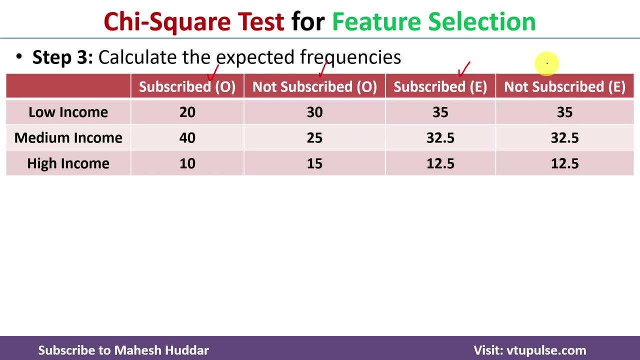 of medium income given, not subscribed is equal to 32.5. expected frequency of high income given, not subscribed, is equivalent to 12.5. here now we need to write it in the table. this is how the table look like. we have already uh written these two things. i have just added the expected. 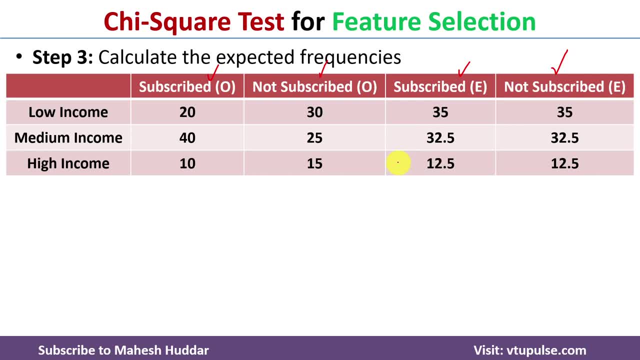 subscribed and not subscribed frequencies here. now what we need to do is we need to calculate the chi-square value in the fourth step here. this is the formula to calculate the chi-square value. that is, chi-square is always equivalent to summation of observed frequency minus expected. 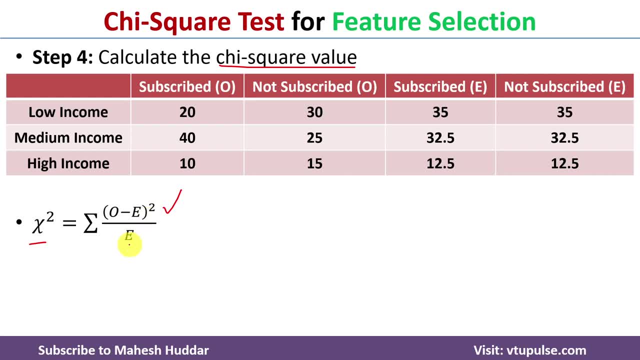 frequency bracket square divided by expected frequency. here chi-square is equivalent to. you can notice here the observed frequency for low income is 20 whenever it is subscribed and expected frequency for low income is 35 whenever it is subscribed. so what we need to do, 20 minus 35 bracket square divided by 35, that is. 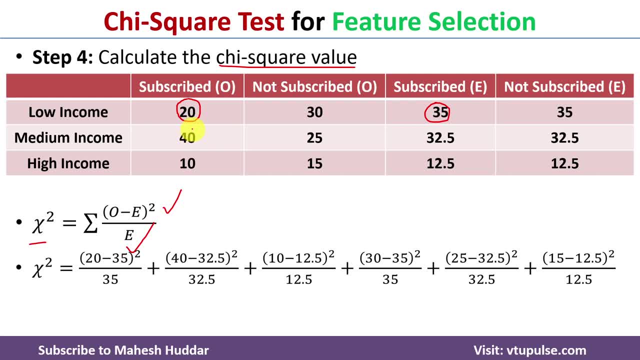 what i have written here. similarly, for medium income, the observed frequency when it is subscribed is 40 and uh expected frequency when it is subscribed is 32.5. so 40 minus 32.5 bracket square divided by 32.5 here. similarly, 10 minus 12.5 bracket square divided by 12.5 with respect to: 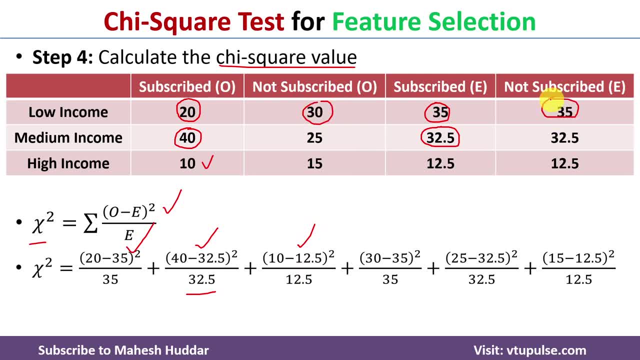 non-subscribed. 30 minus 35 bracket square divided by 35. 25 minus 32.5 bracket square divided by 32.5 here. and 15 minus 12.5 bracket square divided by 12.5 here. once you solve this equation, chi-square. 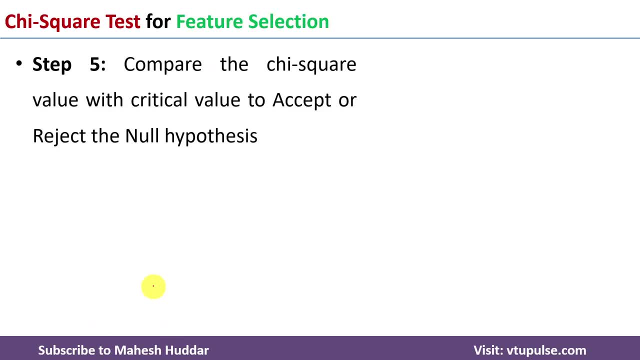 value is equivalent to 11.6 in this case. now what we need to do is, in the fifth step, we need to compare the chi-square value with a critical value to accept or reject the null hypothesis. now the question comes in front of us: how to calculate the critical value here to calculate: 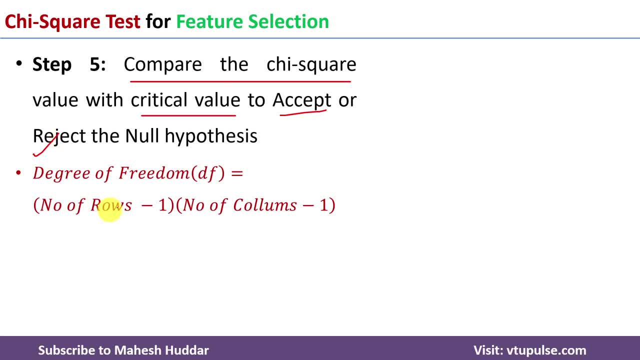 the critical value. first we need to calculate the degree of freedom. degree of freedom is always equivalent to number of rows minus 1, multiplied by number of columns minus 1. here, number of rows in this case is 3, because there are three possibilities. are there like low income? 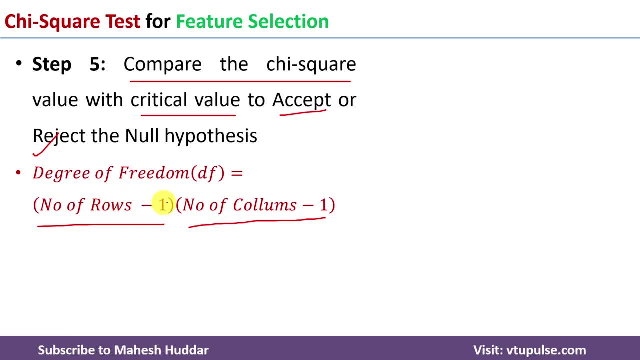 high income and medium income. so 3 minus 1 is equivalent to 2. here number of columns are 2 subscribed and not subscribed. so 2 minus 1 is equivalent to 1 in this case. that is, 2 multiplied by 1 is equivalent to 2. here the degree of freedom is equivalent to 2 in this. 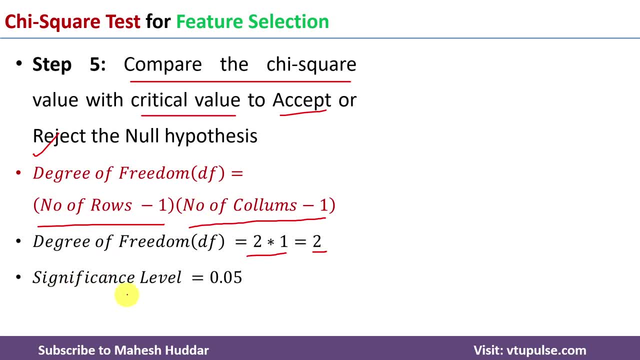 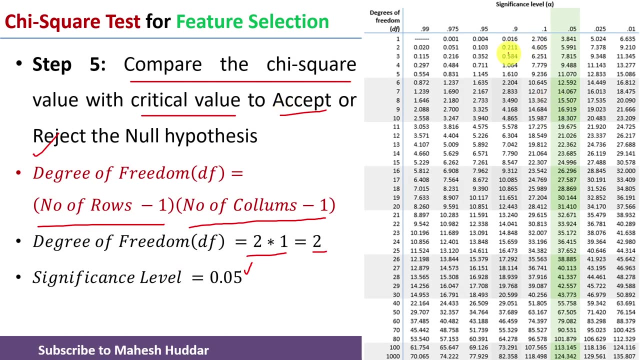 case, one more variable is required. that is known as significance level. by default it will set to 0.05 in chi-square test for feature selection here. now, once you know the degree of freedom and significance level, we can easily calculate the critical value using this table here that: 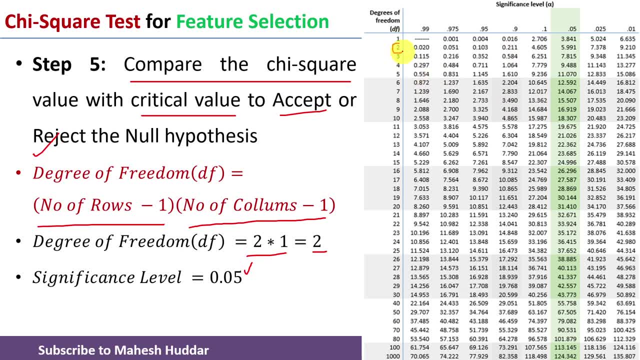 is a chi-square table. the degree of freedom is equivalent to 2 here and the significance level is equivalent to 0.05. the value for this one is 5.991 in this case. so this is what is the critical value for the given degree of freedom and significance level in this case. 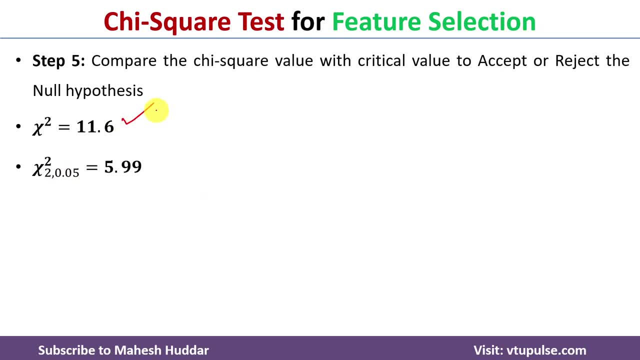 now what we have done. we have calculated the chi-square value. that is equivalent to 11.6 and the critical value is equivalent to 5.99 in this case. now we need to compare these two things. if the calculated value is greater than the critical value, 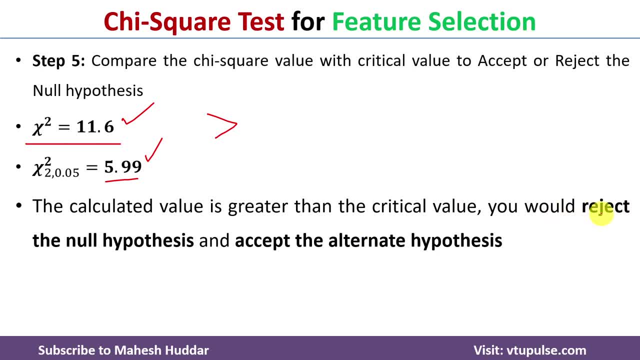 then the null hypothesis will be rejected. so the null hypothesis is rejected means what the alternate hypothesis will be accepted in this case, what null hypothesis is. the given feature is not relevant to the target here, so that is what the null hypothesis is. if you reject the null, 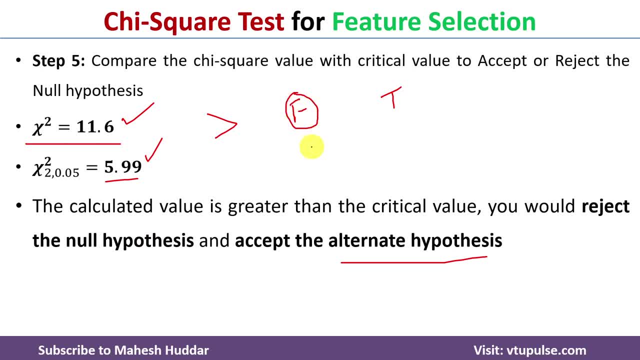 hypothesis. what is the meaning of that one? the given feature, that is, the income, is relevant to the target in this case. so that is what i have written here. the income level is relevant feature for predicting the subscription status in this case. in this case, i have shown for only one. 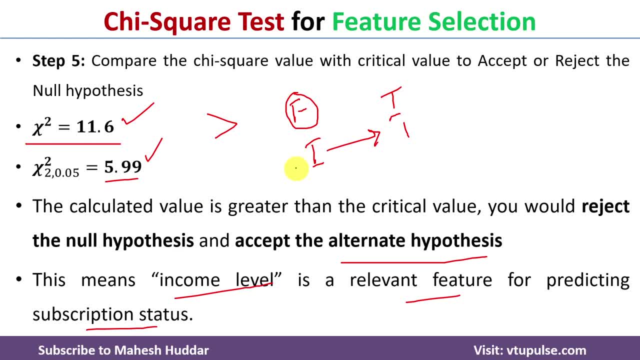 feature. the same thing has to be done for all features in the given data set, and then we need to check whether the given feature is relevant or not relevant in this case. so this is how we use the chi-square test for feature selection in machine learning. i hope the concept is clear.